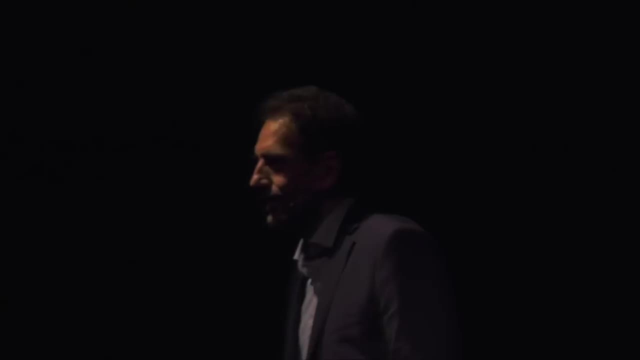 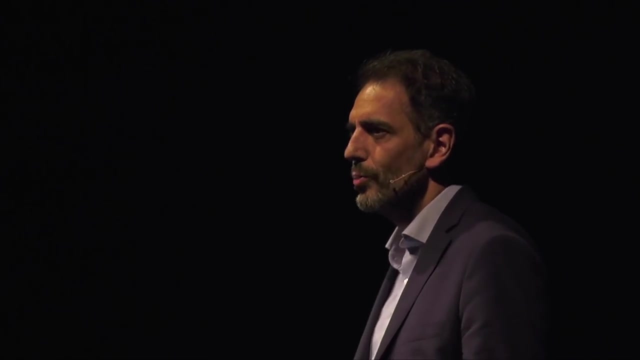 of data every two days. That's a huge amount of data, But the good news is that the technology today enables us to handle, process and analyze all the data that we need to be able to do the work that we need to do. 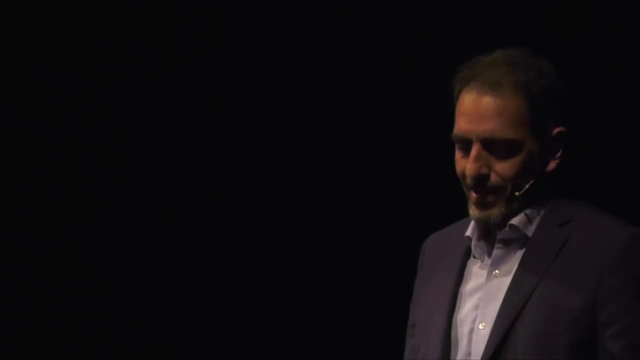 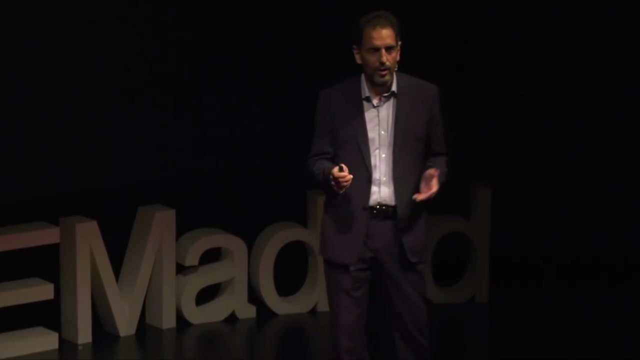 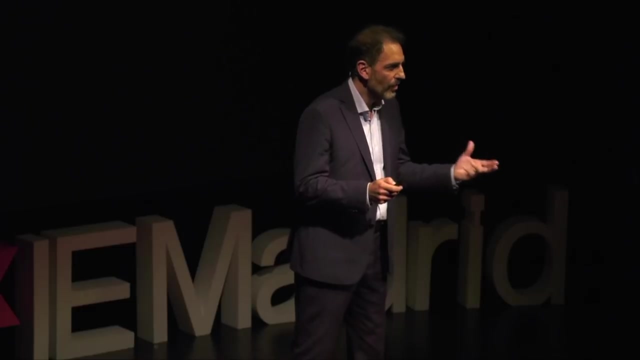 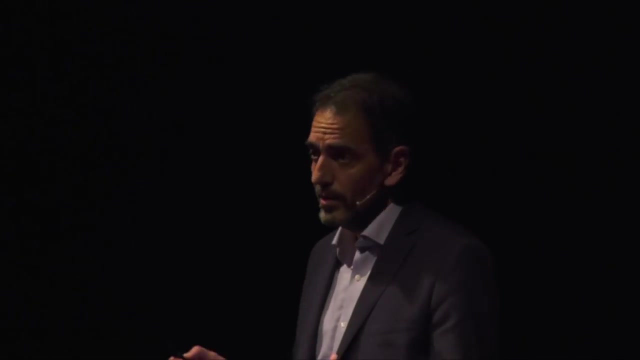 With the help of artificial intelligence, of machine learning, big data is being used for a number of things: for better profiling users, for doing personalized recommendations, for improving healthcare and diagnosis, for predicting political revolution, preventing crime and even creating a new world. 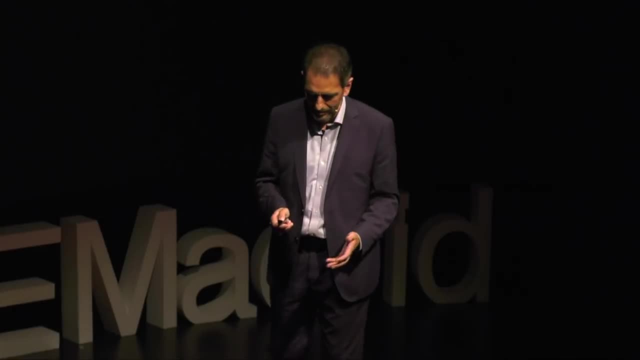 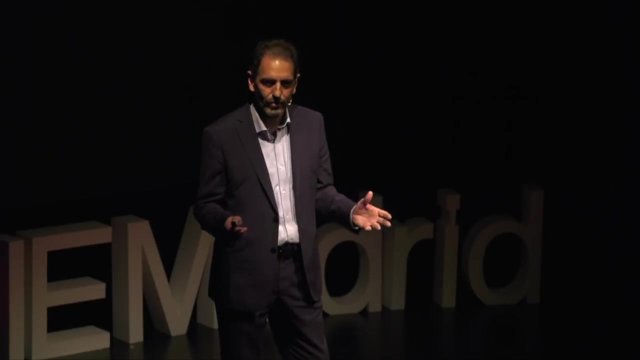 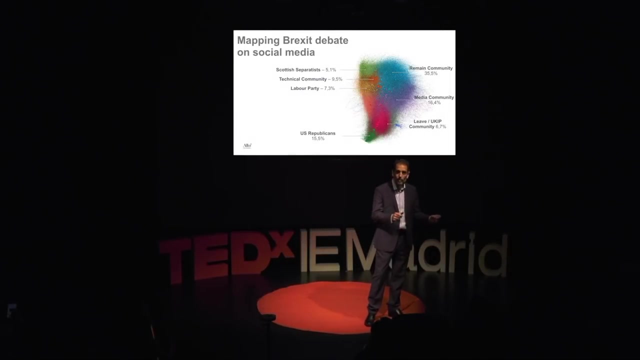 It's clear that big data enhances human potential. At Altodata Analytics, we help large organizations drive actionable insights from all kinds of data to make a difference. And then, when there's a social debate, like in the months after the Brexit, we can analyze. 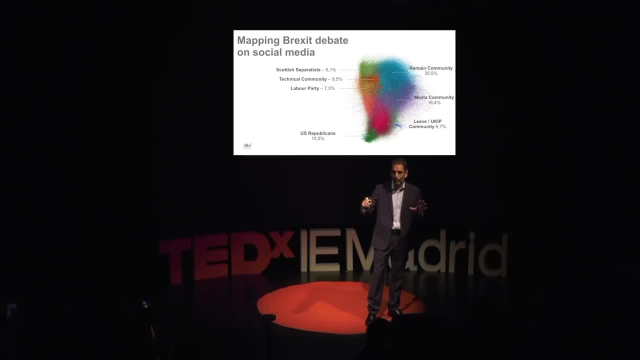 the data and understand and map where the social debate happens and what communities were created. We can see how the data is being used. We can see how the remainers were opposed to the lead community. how the media community was seated in the middle, kind of neutral. how there was a technical community who were 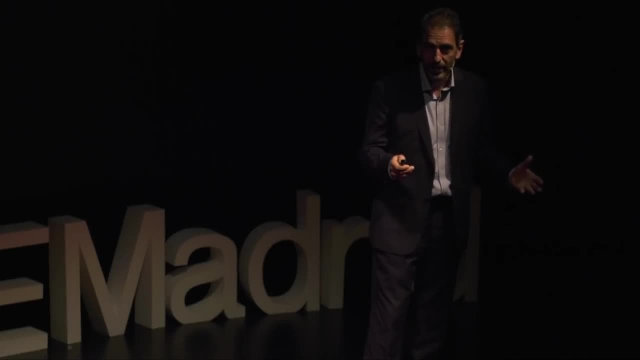 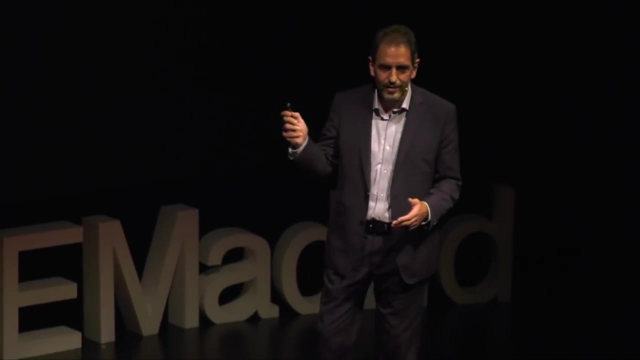 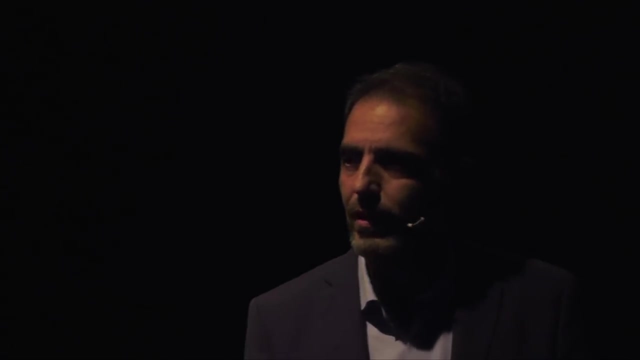 the people talking about the economic and social and political implications of the Brexit that were closer to the remainer community. We can see also other communities emerging, like the Scottish, the separatist Scottish, which are closer to the status of the remainers, or how the US Republicans appear more in. 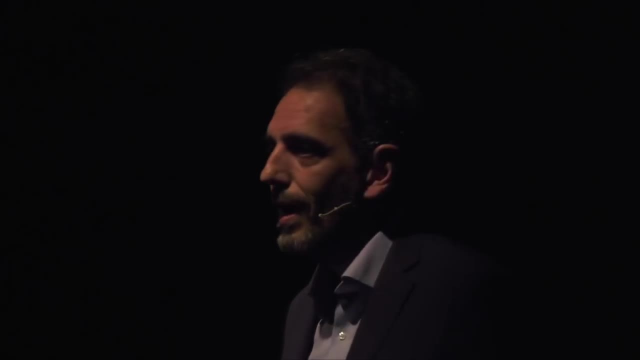 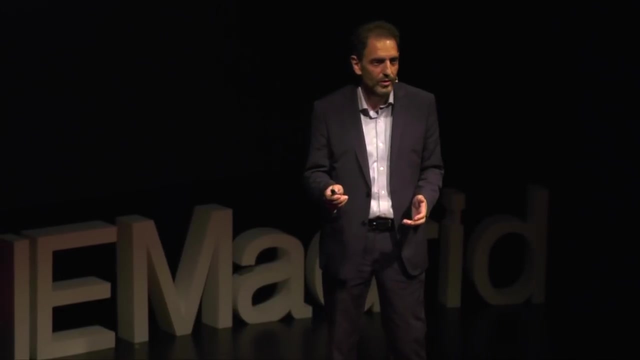 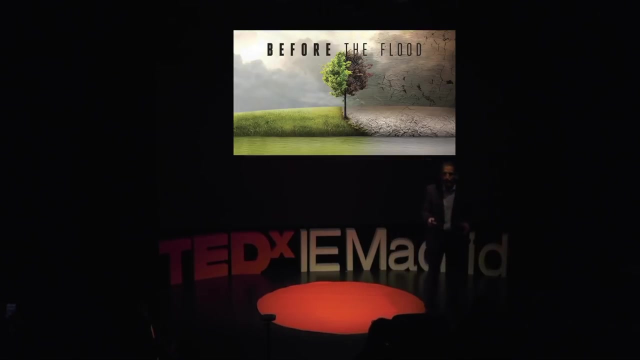 the side of the Brexit. We can also analyze and understand who were the most influential people in the debate and how the media itself was positioned, and even predict what agendas will prevail. And as for a movie, we can analyze far more than what the critics say. 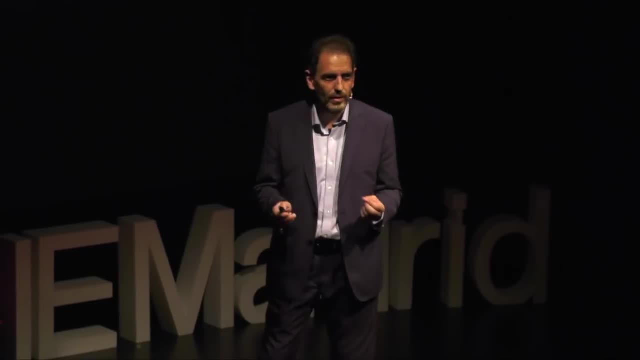 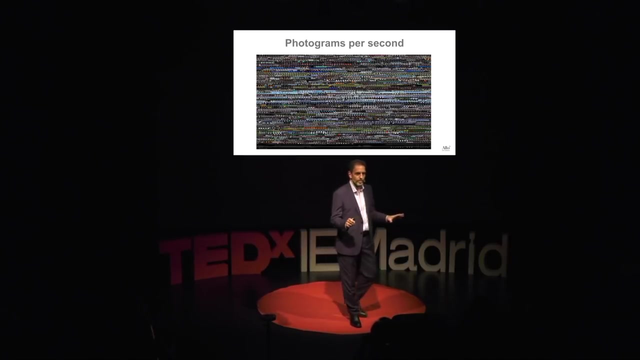 In Leonardo DiCaprio's documentary The Greatest Showman. the film is based on the documentary Before the Flood, a documentary to raise awareness about climate change. What we did is we captured all the photograms so that we could analyze and understand how. 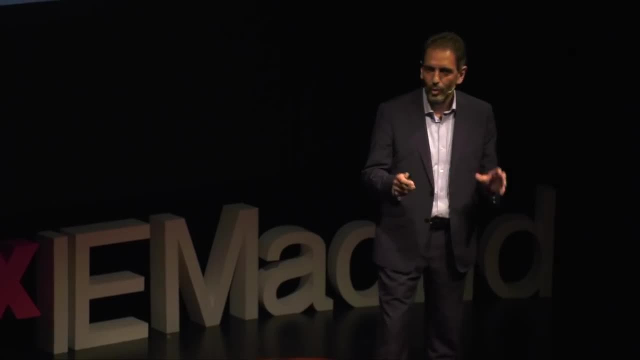 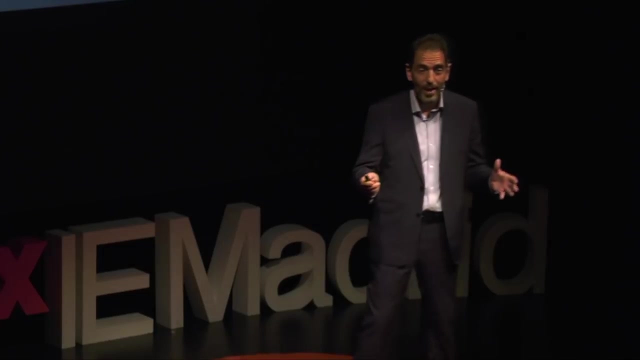 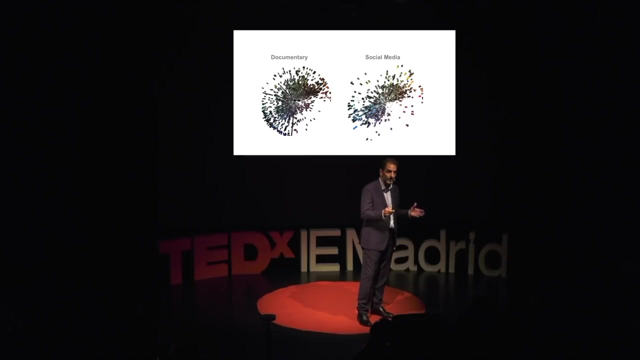 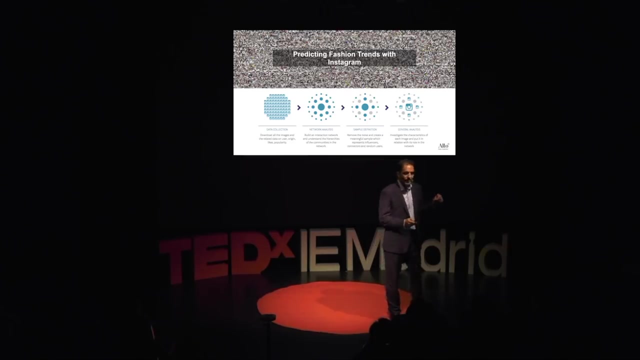 many of them DiCaprio appears and how many of them policymakers appear, to understand and determine which were the aspects of climate change that triggered more debate, or we can understand as well which of the visual sequences were shared, Thank you. And in fashion? we can even predict trends in fashion by analyzing the photographs that 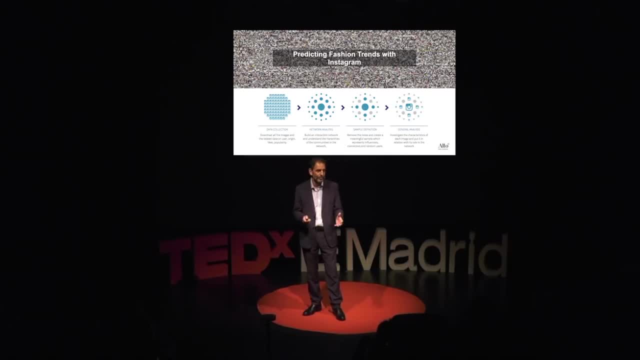 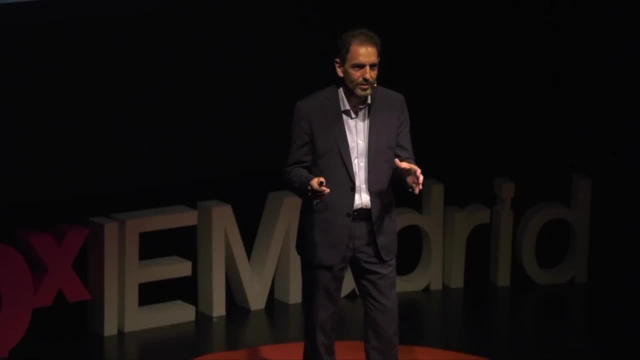 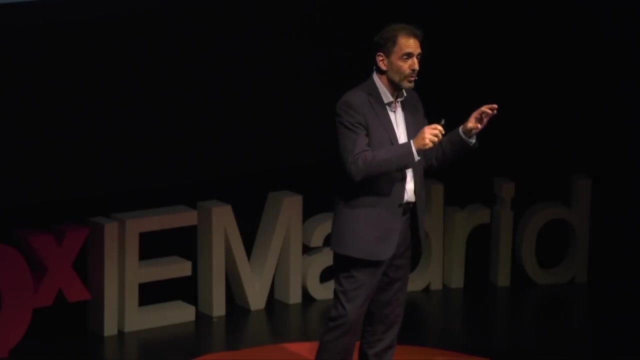 people share in Instagram with hashtags such as Artfeed of the Day. We collect all the hundreds of thousands of photos. Then we can analyze the underlying influence of people sharing those photographs because we can see who interacts with who and then see what patterns emerge in the photos that 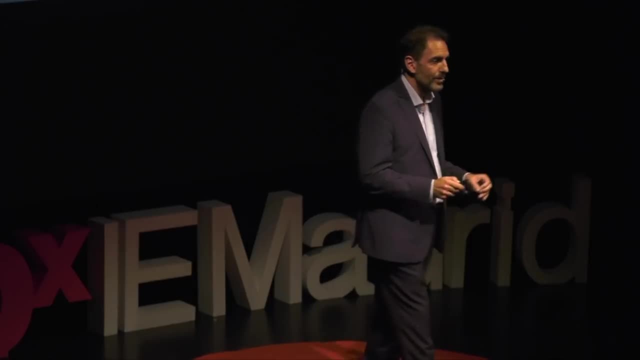 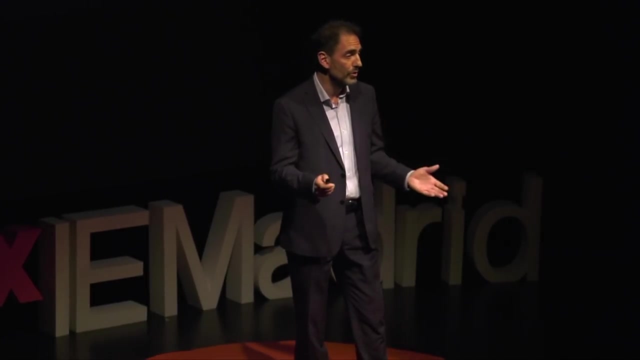 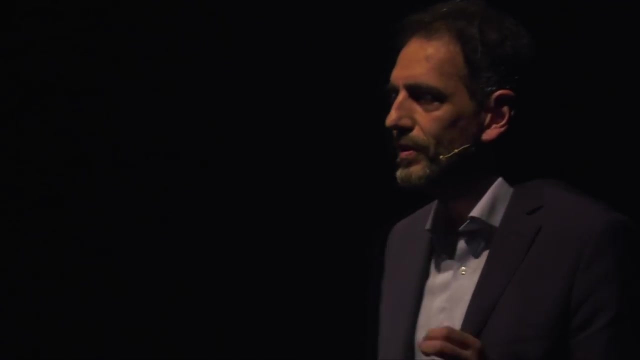 most influential people share. It's a paradigm shift where we used to make decisions based on intuition and guesswork. Now we can manage this on evidence. We can move to data-driven decisions. Management guru Peter Drucker said that you cannot manage what you cannot measure. 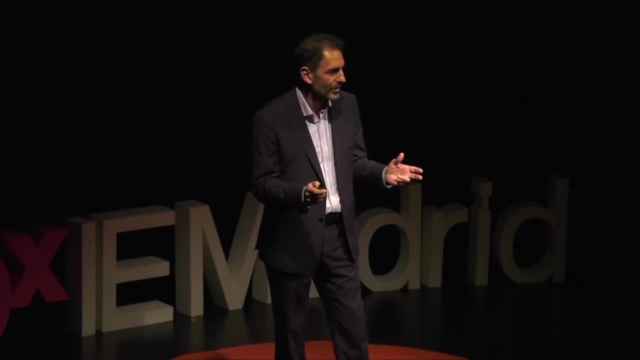 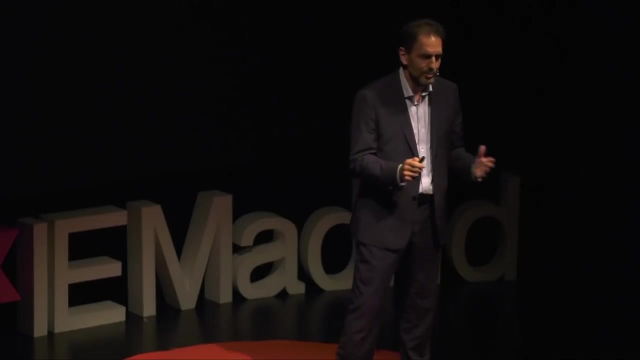 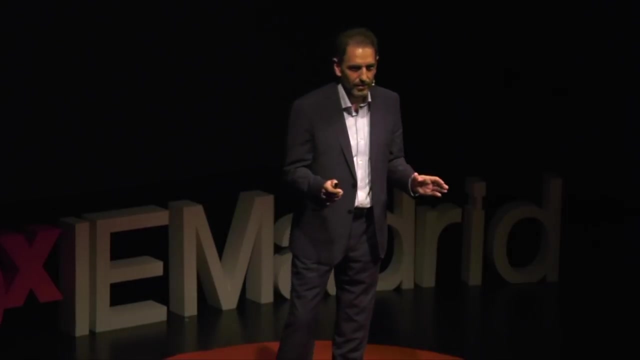 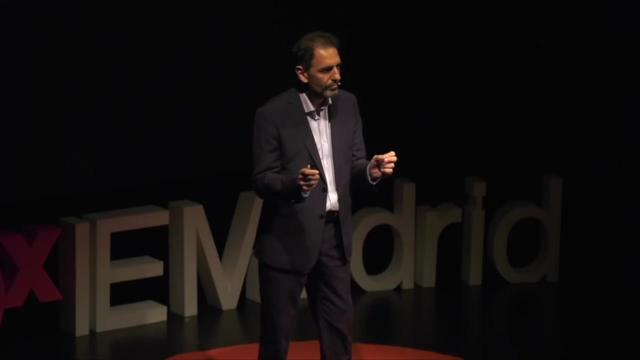 Now there's no excuse. You can measure and you can manage. Without the help of artificial intelligence, machine learning and all the big data technologies, we would not be able to handle all this data revolution. But still, the most important element in driving insights out of data is what makes a data scientist. 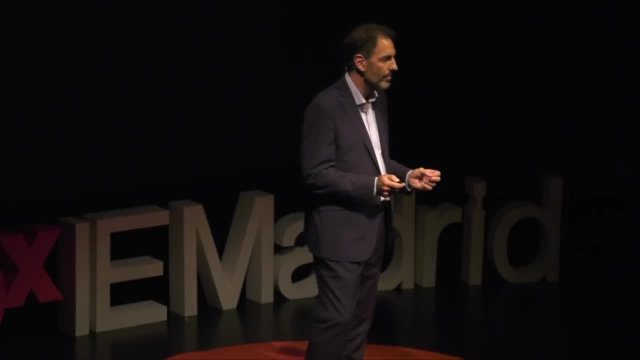 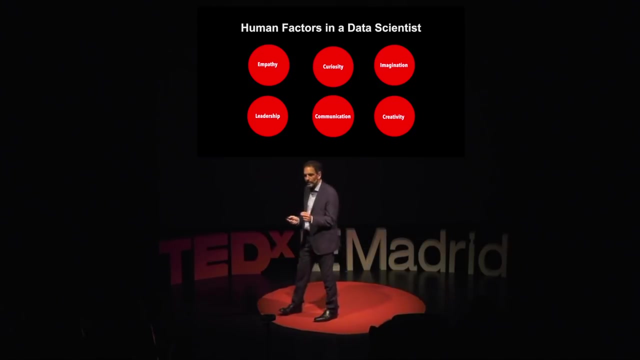 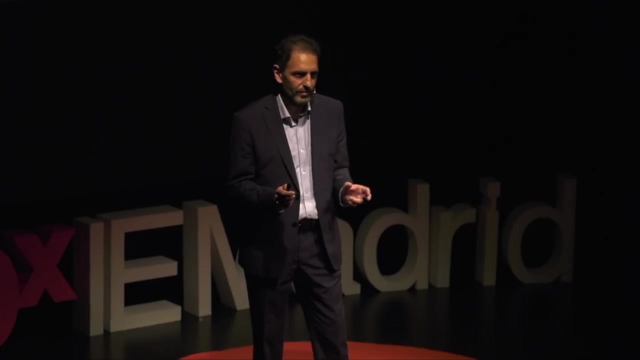 irreplaceable. It's a human factor. The key to turn data into insight lies in what we can do that machines can't. Curiosity: We all have access to Google- more than billions of data points in Google- But it's your curiosity that? 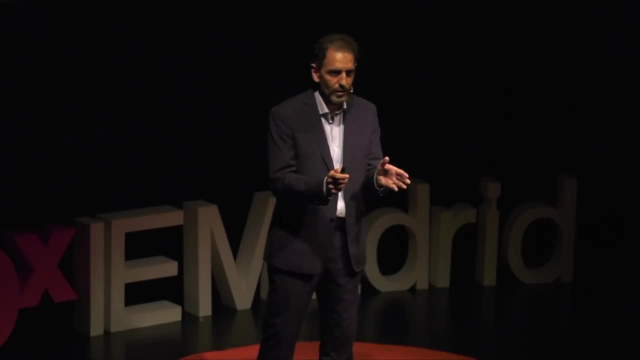 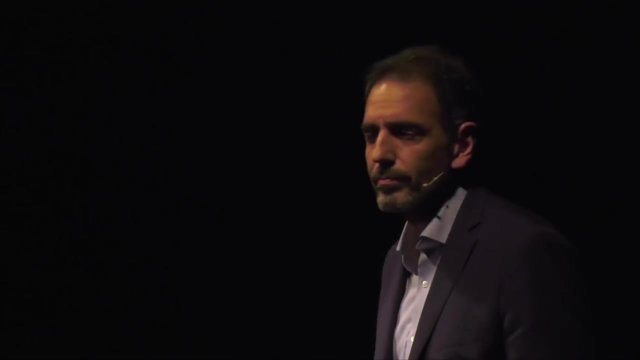 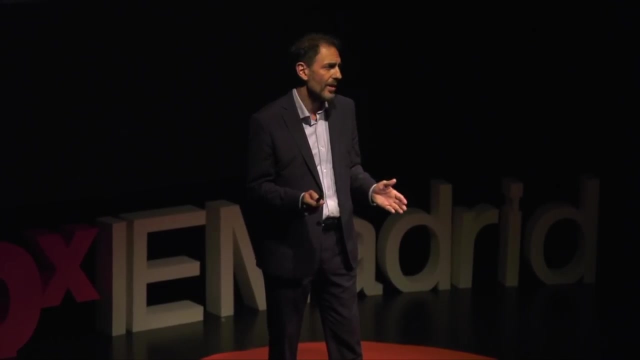 determines what you will learn, what you will search for and therefore also what you will filter and how you will discover what's relevant to you: Empathy- Empathy is the cost to connect with others and to understand what other people need, Henry Ford said. 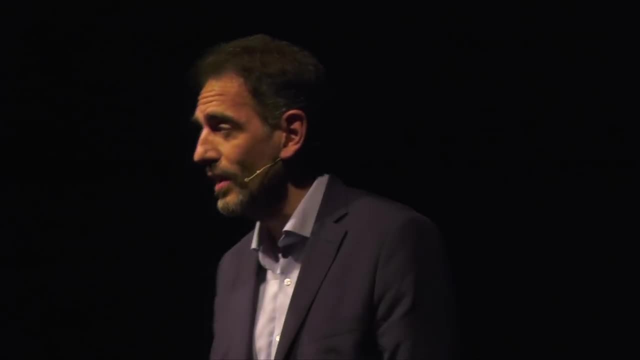 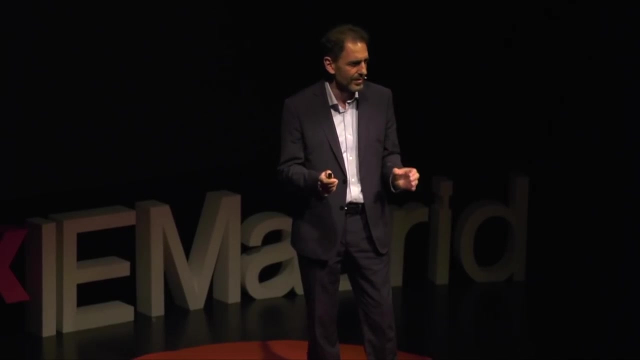 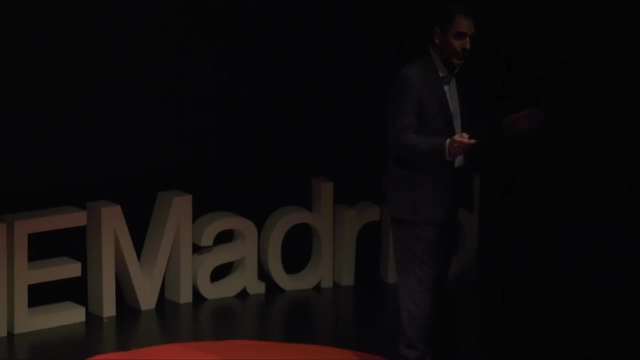 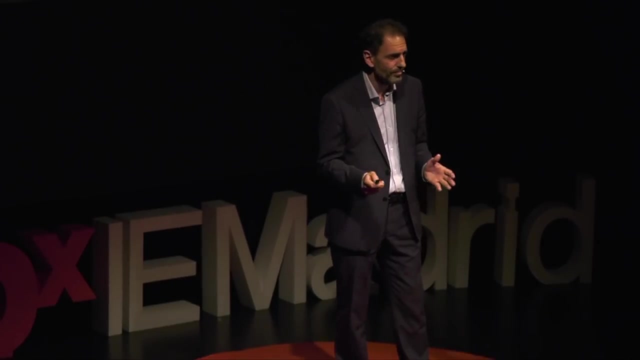 True That if I would have asked people what they wanted, True they would have said faster horses. imagination is the key to visualize what doesn't exist yet creativity. creativity is the key to invent and articulate solutions to solve problems. communications is the key to persuade to. 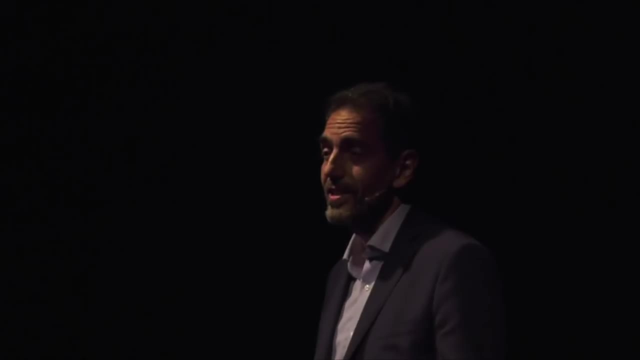 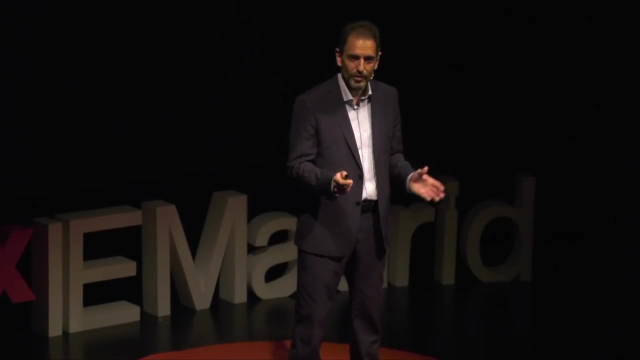 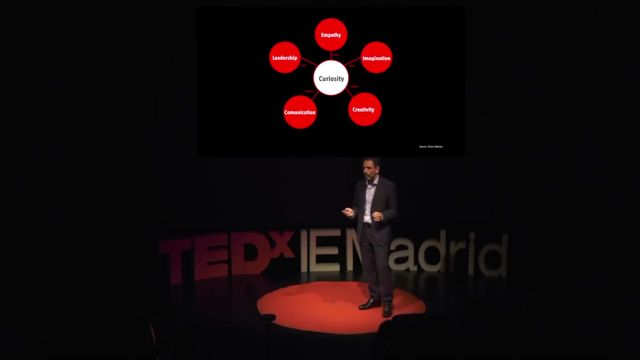 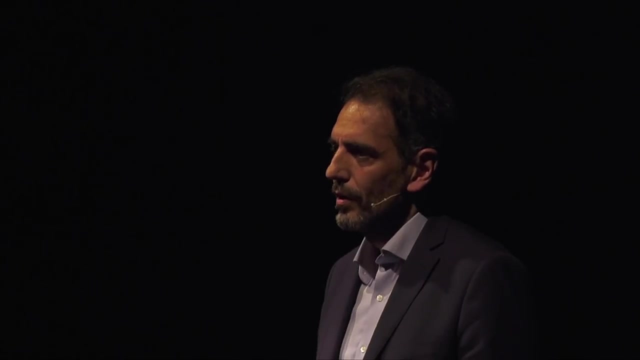 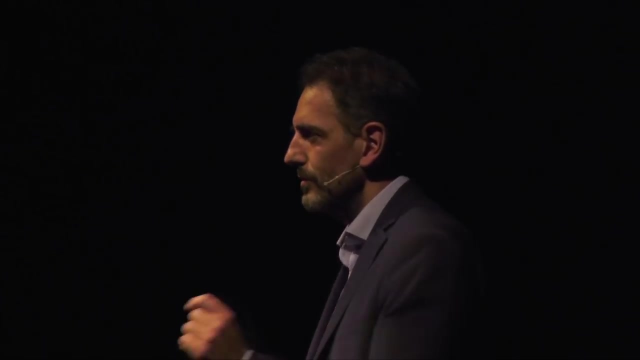 influence and to spread ideas that create change. and leadership is the key to step up and move all these people to action. and at the center of them all is curiosity, because it is curiosity for emotions that drives empathy, it is curiosity for ideas that drives imagination, it is curiosity for solutions that drives creativity. it 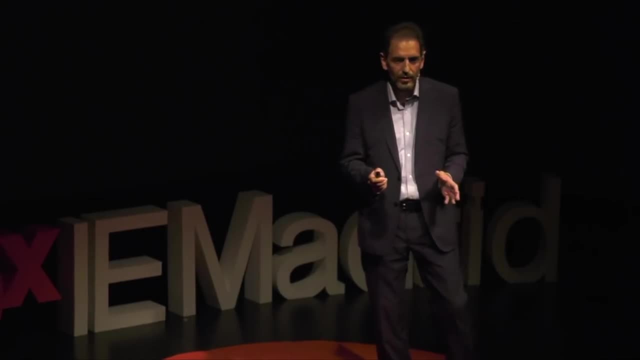 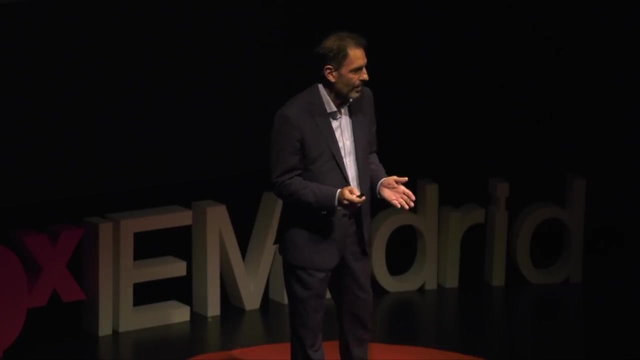 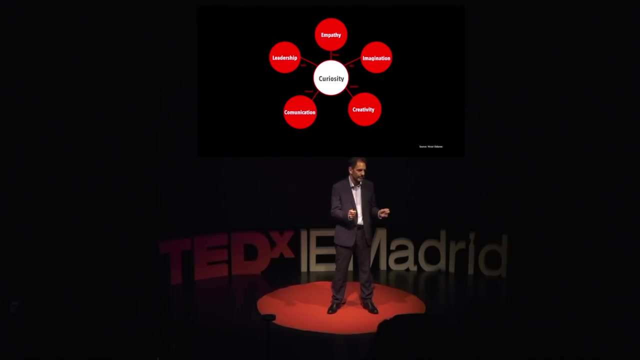 is curiosity for influencing that drives communications and it is curiosity for results that, in the end, drives leadership. the most important skill of a data scientist is asking the right question to data, the curiosity of a data scientist to ask that the right question, those right questions. to iterate, to understand human issues, to imagine the. 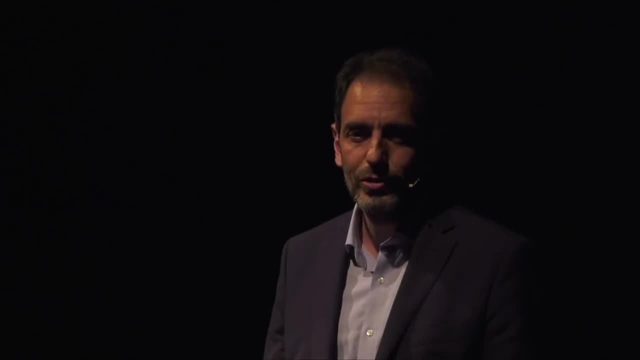 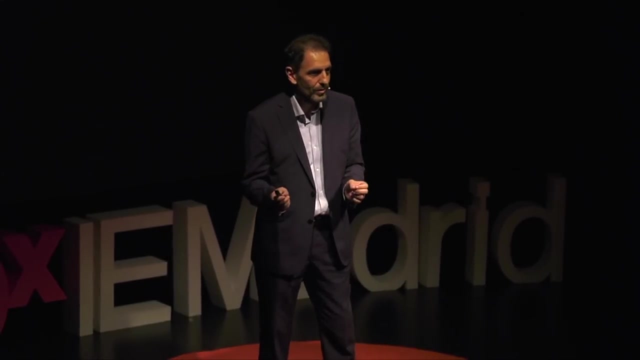 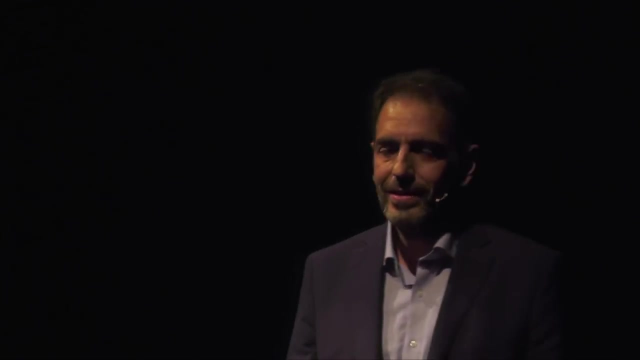 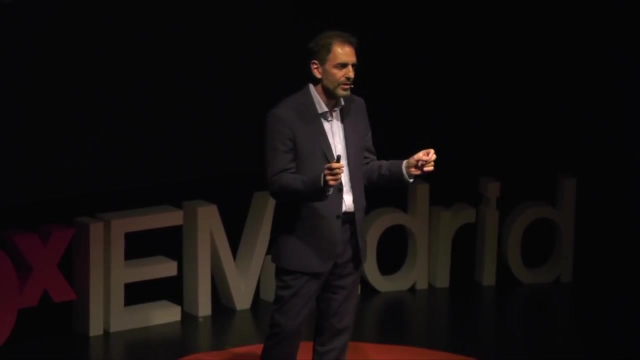 possibilities to create an articulate solutions to convey the message and insights, with the right visuals to make them actionable. those are the key elements that turn data into something meaningful. it's a set of skills that no artificial intelligence can match, yet it's. it is at the intersection of technology and liberal arts where magic 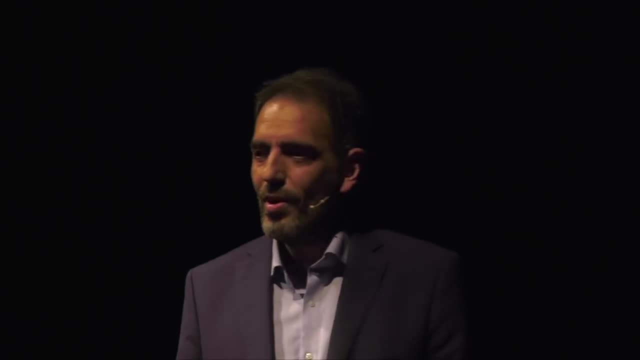 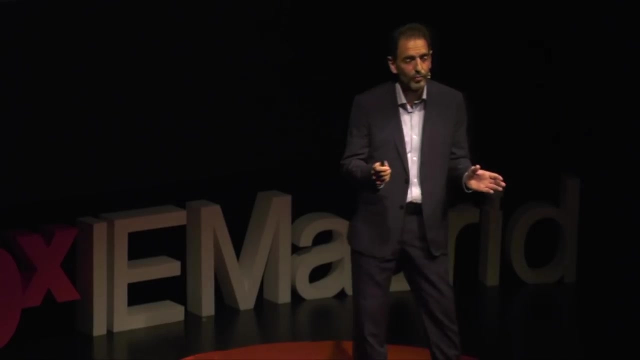 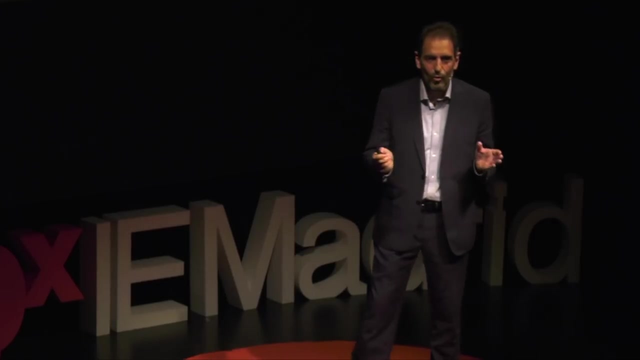 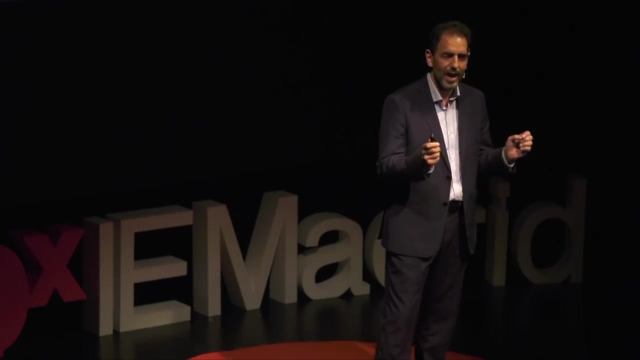 happens if the Renaissance of the 14th and 17th century was a cultural force that drove humanity out of the Middle Ages and into the modern era? the big data Renaissance is already unveiling endless possibilities to push humanistic the human race forward with the power of data. it is up to us to imagine what data